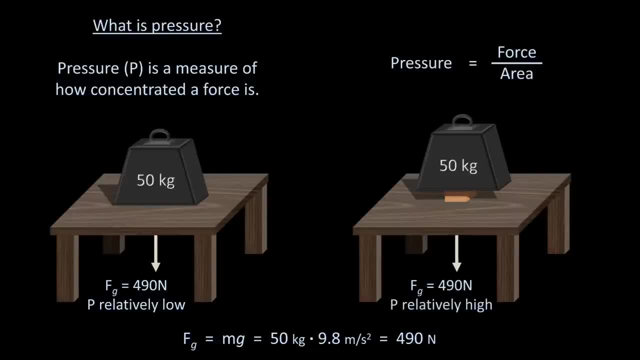 will be relatively high. In fluid mechanics, instead of one solid object imparting pressure against another solid object, we have a fluid imparting pressure against a solid, But the concept of a force per unit area is the same. When talking about fluids, there are a number of different types of pressure. that one 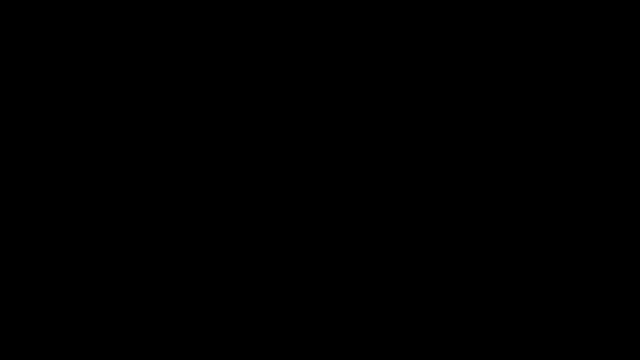 can discuss. However, the most fundamental and important of these is something called the hydrostatic pressure. This is the pressure present within the fluid when it is at rest. It acts equally in all directions and it acts at a right angle to any surface that is in contact with. 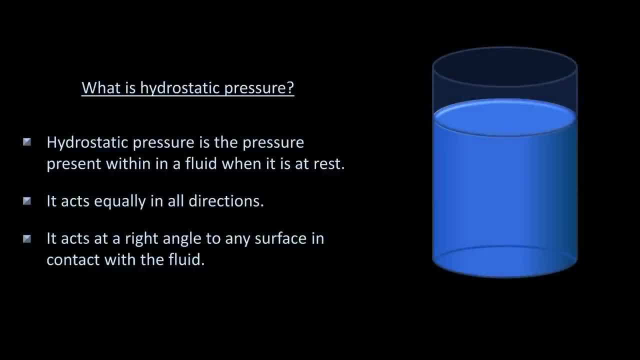 the fluid. So if we have a glass of water at a given level within the water, the hydrostatic pressure, which is a result of the water and the surface unwielding, represents the heat as we Fold. The statistical meaning of the idea is that it increases the pressure of cuidon, Which 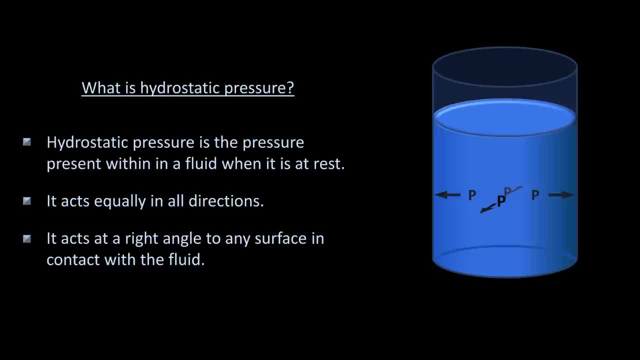 weight of fluid above it acts on the side of the glass equally in all directions, Since pressure is the force divided by area. if the pressure was somehow unequal, it would mean the forces on the glass were unequal, which would consequently result in the glass 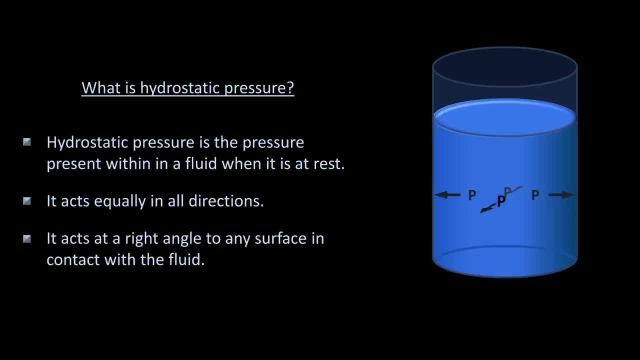 of water moving And of course we know that a glass of water at rest does not start to slide laterally on its own. As another example of this, imagine taking a playing card and submerging it vertically into the water. The hydrostatic pressure in the water will act at a right angle to any surface in contact. 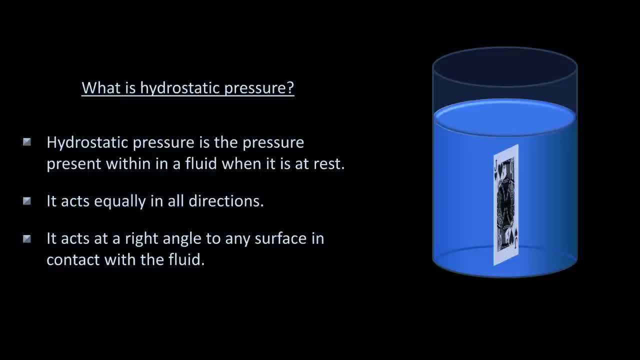 with the fluid. That means that there is a right side of pressure pushing on the left side of the card and a left side of pressure pushing on the right side of the card. As these forces are equal, the card will not spontaneously move in either direction. 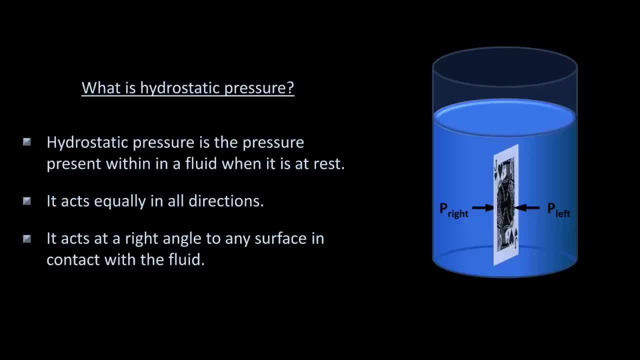 Keep in mind, however, that just because there is no net lateral force on the card caused by the hydrostatic pressure does not mean there is no net force on the card. From the last lesson we know that there is still the card's weight and the card's. 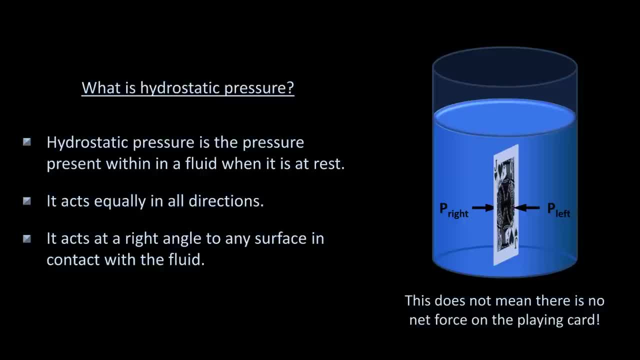 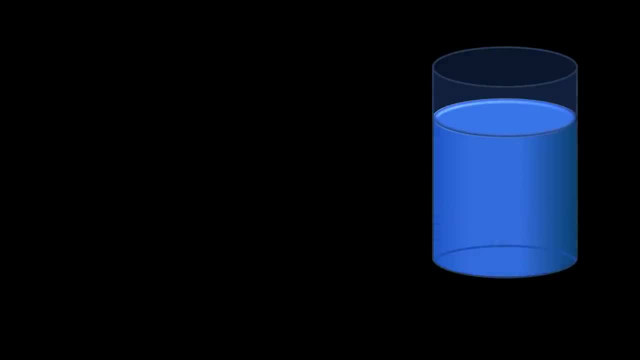 buoyancy. So unless the card is exactly the same density as water, it will still move either up or down within the water once released. Is there any way to quantify the hydrostatic pressure? Common experience might tell us that the pressure in fluid increases at increasing depth. 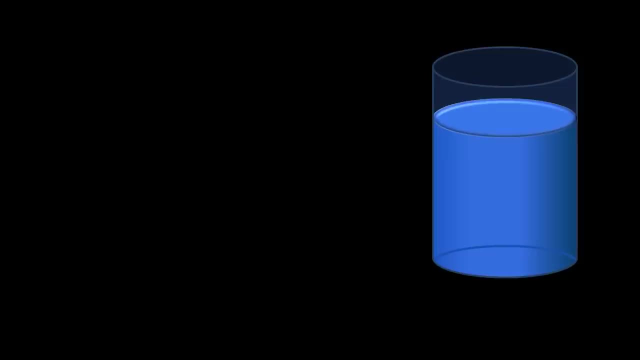 For example, when you jump into a deep swimming pool. If you've ever dived deep Down underwater, you've probably felt the pressure increasing as you go down deeper and deeper. Quantitatively, this pressure increase can be calculated with this equation: 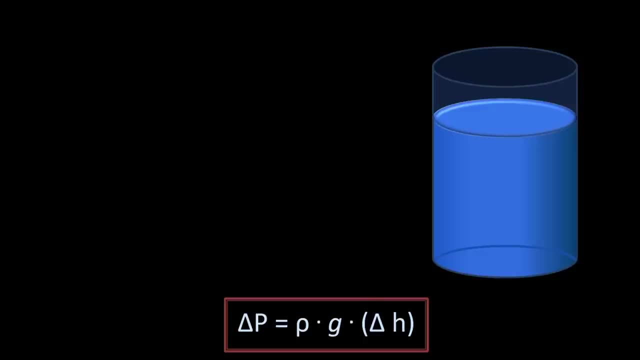 The difference in pressure between two points is equal to the density of the fluid times. little g times the difference in vertical height between the two points. In the case of the glass of water here, if we were interested in the pressure at the bottom, the two points we would use would be its bottom and top. 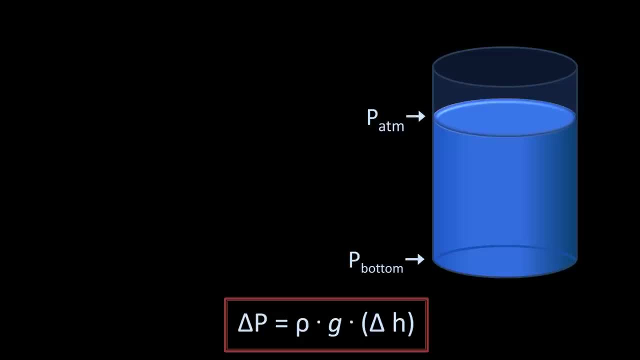 The pressure at the top is equal to atmospheric pressure and the difference in vertical height is just the depth of the water. To refer back to the last lesson on Archimedes' Principle and buoyancy, some of you might realize that the buoyant force on a submerged object, which we said was equal to density. 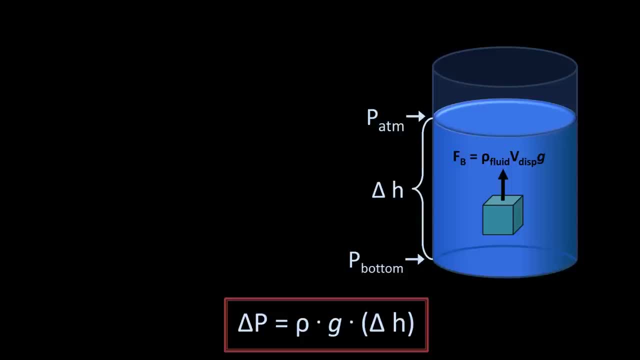 of the fluid times. volume of the displaced fluid times. g is simply a manifestation of the difference in hydrostatic pressure that's acting upwards on the bottom side of the object and the hydrostatic pressure that's acting downwards on the top side of the object. 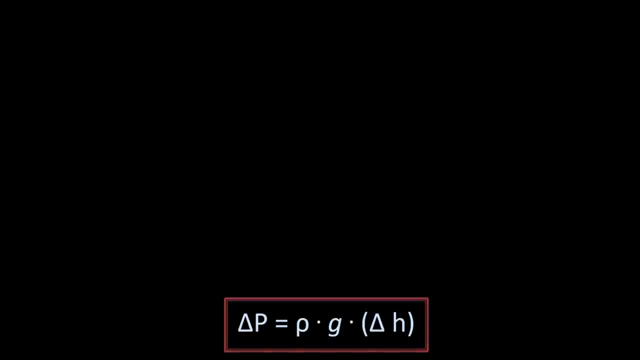 An interesting consequence of this hydrostatic pressure equation, which may or may not be immediately obvious, is that the pressure at any given depth is independent of the shape of the container or the path that the pressure must be transmitted along. For example, I could have a collection of rare and exotic jellyfish that I want to display. 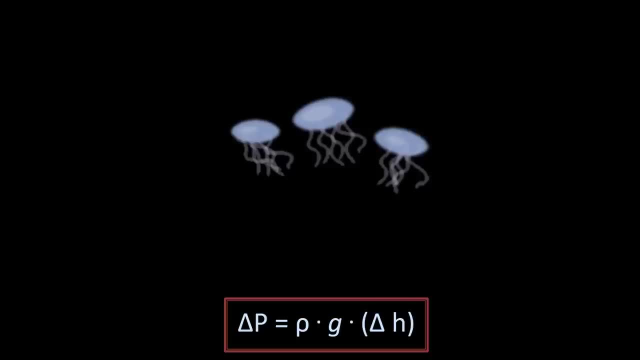 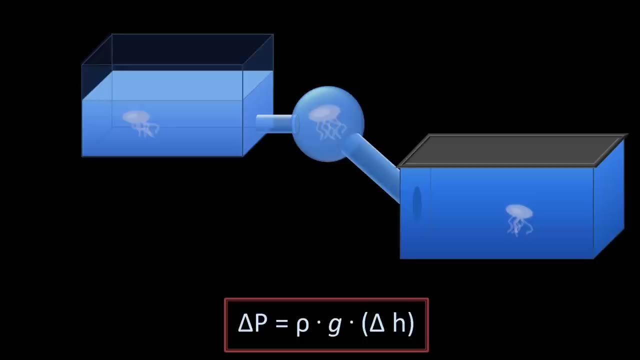 in my home, but to highlight their uniqueness, maybe I want to build an equally unique aquarium system in which to house them. If I wanted to know what the maximum water pressure was at the bottom of the system of tanks, the only thing that would matter is the total vertical distance between the top. 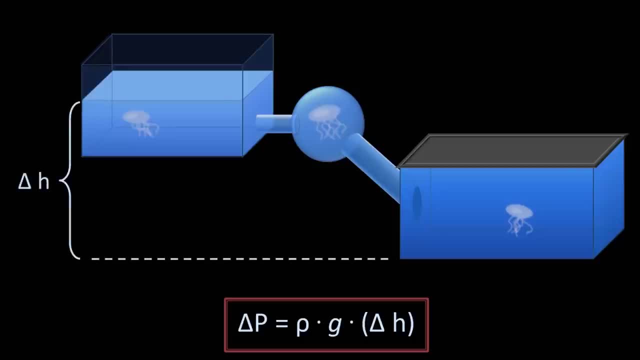 and bottom. The shape of the tanks, the volume of the tanks, the width and length of the connecting tubes are all irrelevant. Also, notice that the lower tank needs a sealed lid. If the lid was not there, the weight of the water in the upper tank would cause the lower. 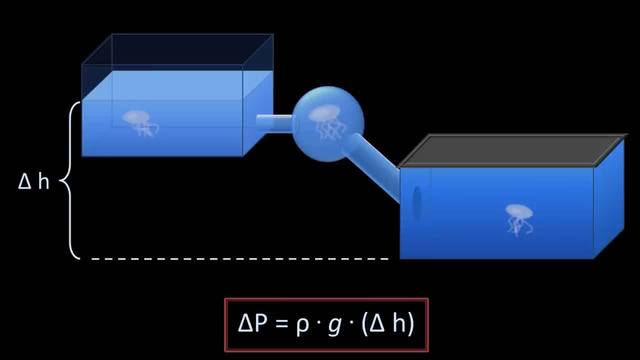 tank to overflow. This is an example of a principle frequently paraphrased: that fluids at rest seek their own level. This means that the surface of any fluid at rest will have the same height above the surface of the earth at all points. Let's look at a quantitative, real world example of hydrostatic pressure. 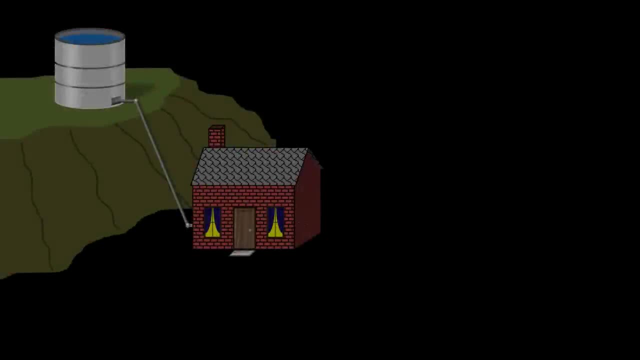 We have a house at the bottom of a hill which gets its water supply from an open, unpressurized water tank at the top of the hill. The water tank is 4.5 meters high. It is 4.2 meters tall, 6.6 meters wide. 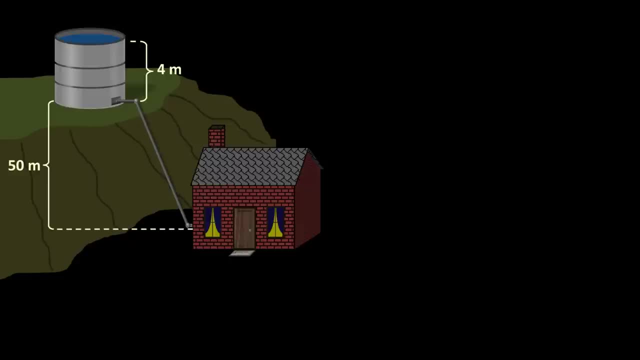 The tank on a higher floor is 40, 4 meters high and full. The base of the tank is 50 meters above the level of the house's faucet. Given these distances, what is the house's water pressure? As we just reviewed, the pressure difference between two points within a fluid system is: 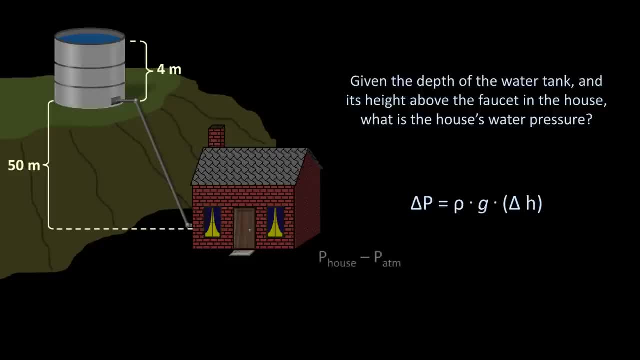 the density of the fluid, times g times the total difference in height between those two points. So we have the water pressure in the house's faucet minus the water pressure at the very is equal to atmospheric pressure. This equals 1,000 kilograms per cubic meter. 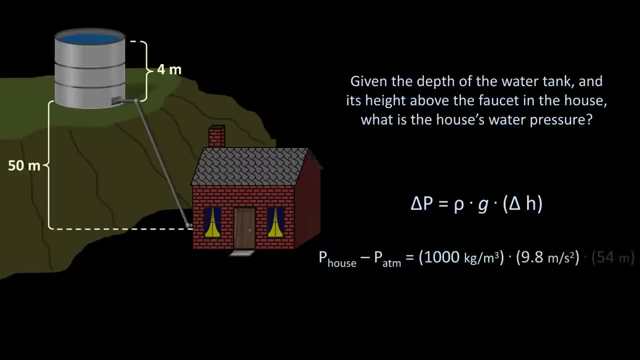 times 9.8 meters per second squared. times the total height of 54 meters, This is equal to 5.29 times 10 to the 5th kilograms per meters second squared, plus atmospheric pressure. The units of kilogram per meter second squared. 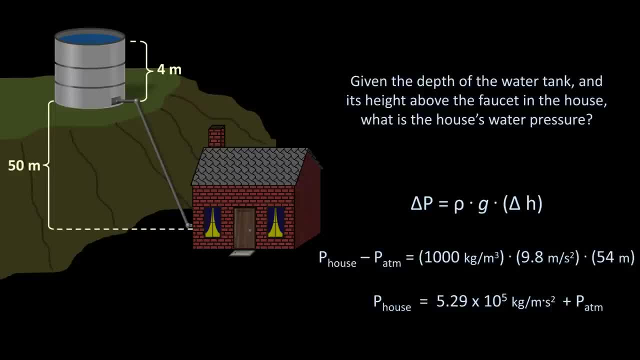 is cumbersome to talk about, so this combination has been defined as its own unit, something called the Pascal, after the French mathematician Pascal, whose name has been attached to a specific physical principle that will be the subject of a future lesson. In addition, this idea of a pressure, 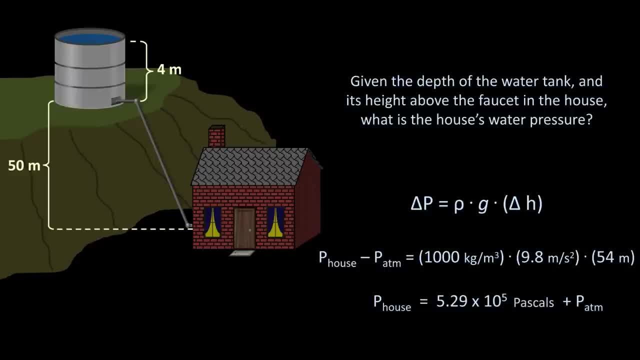 that is equal to some number plus atmospheric pressure, gave rise to the concept of gauge pressure. since atmospheric pressure is essentially equal at both the top and bottom of this type of system, The gauge pressure in this type of situation is the total pressure minus atmospheric pressure. 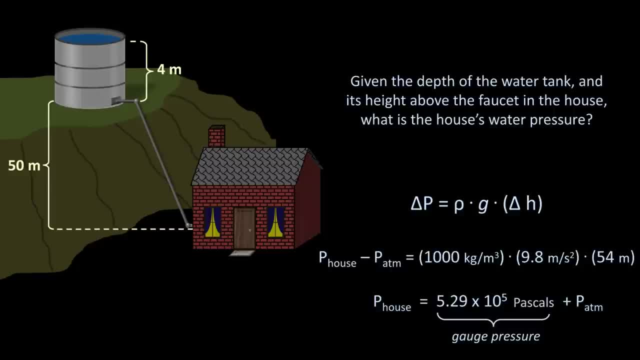 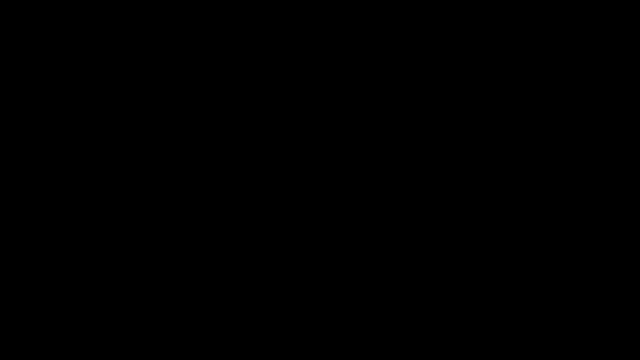 When people refer to the term pressure, in most everyday situations, such as discussing their home's water pressure, whether or not they realize it, the gauge pressure is often to what they are actually referring. That's an introduction to the concept of hydrostatic pressure.